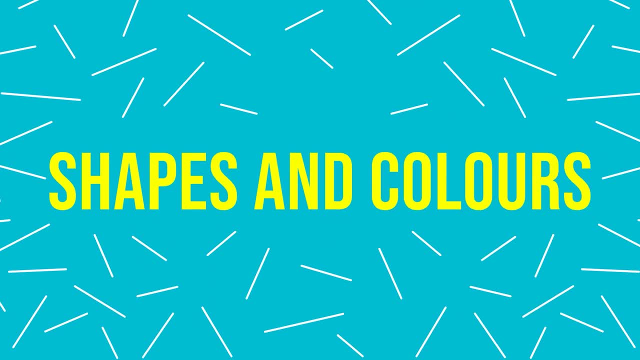 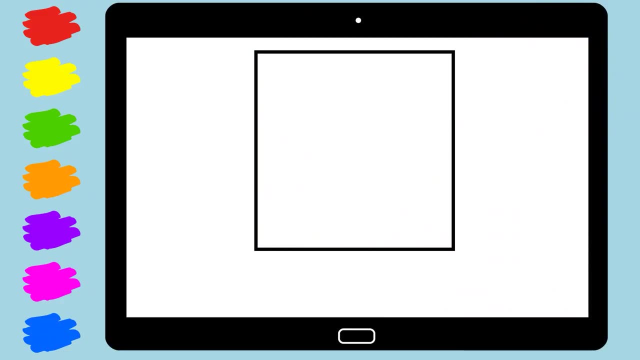 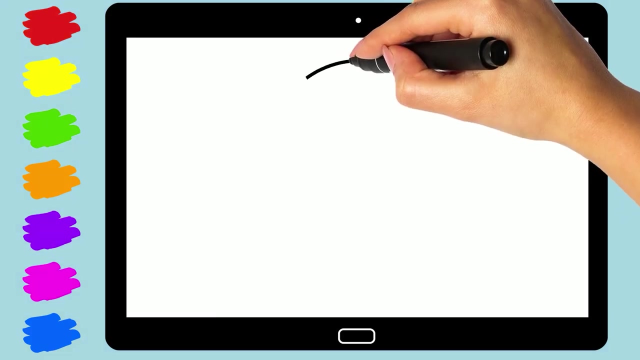 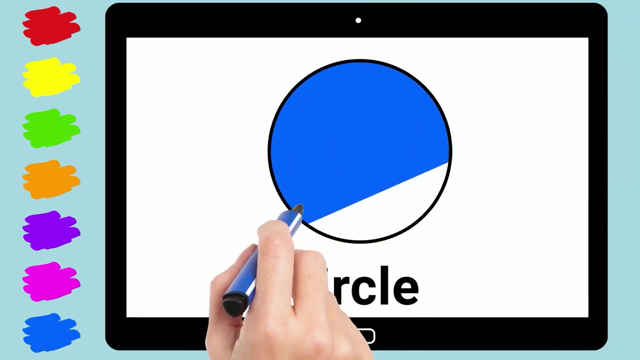 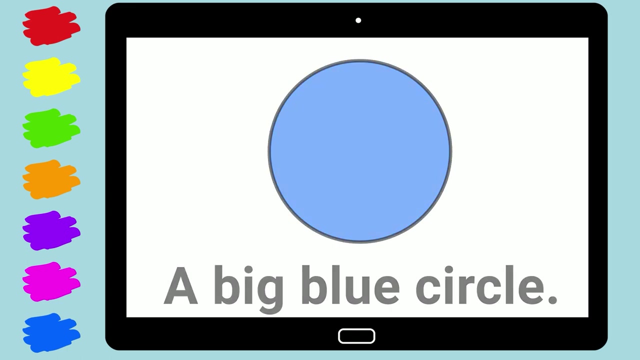 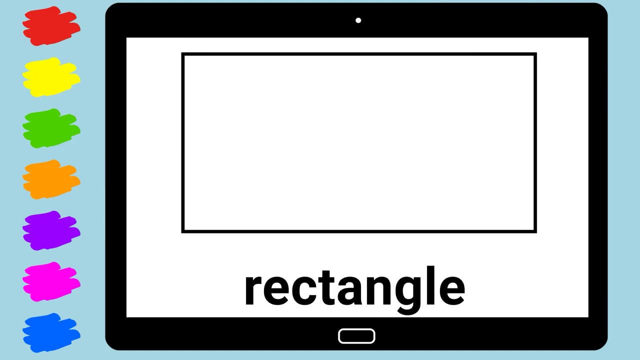 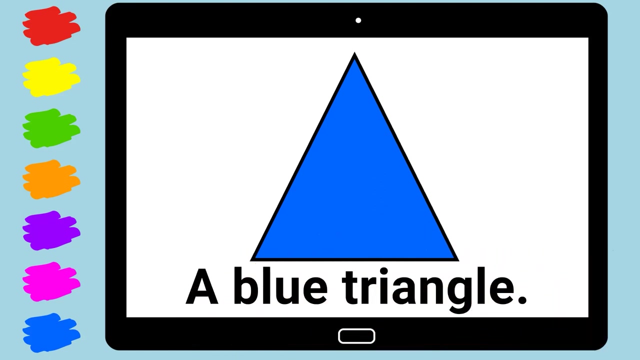 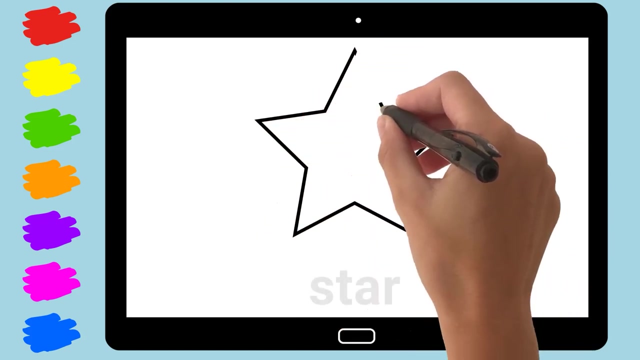 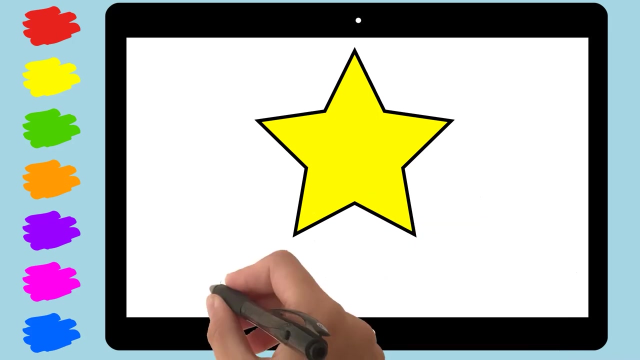 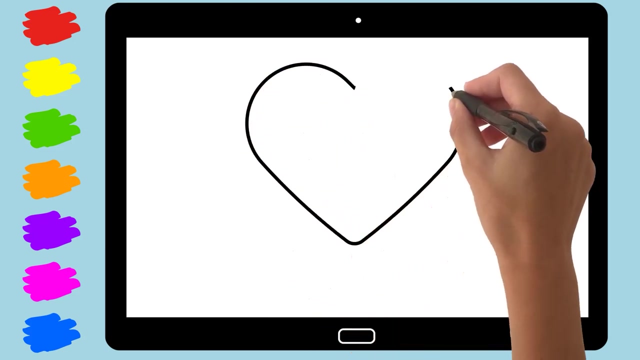 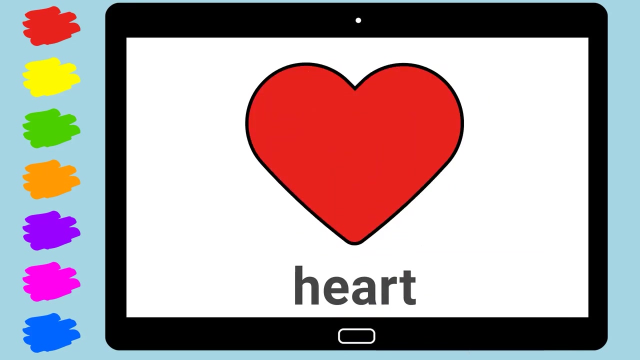 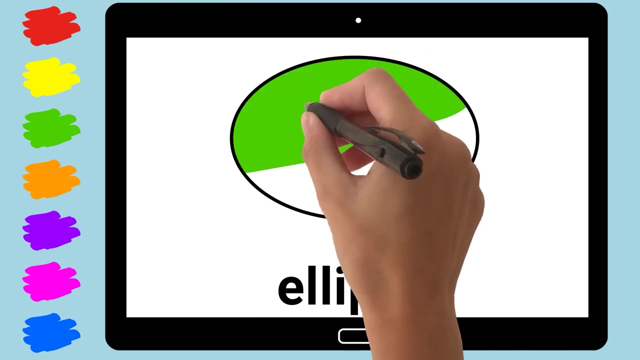 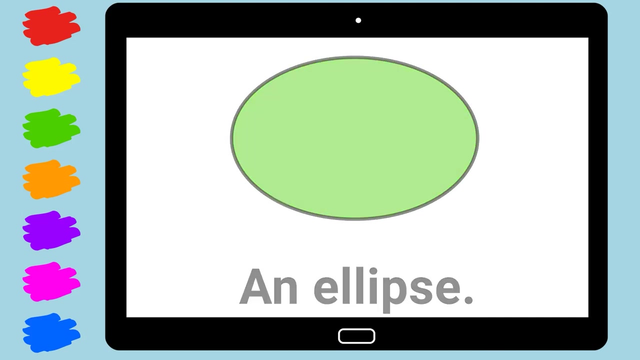 Shapes and colors: Square- A yellow square. Circle, A big blue circle. Rectangle: An orange rectangle. Triangle: A blue triangle. Star: A yellow star. Heart- A red heart. Ellipse- An ellipse. Oval- An oval. 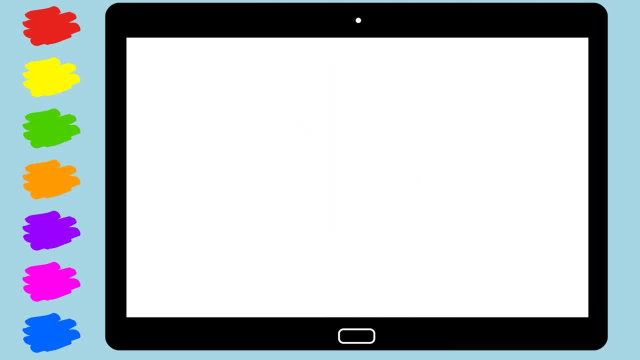 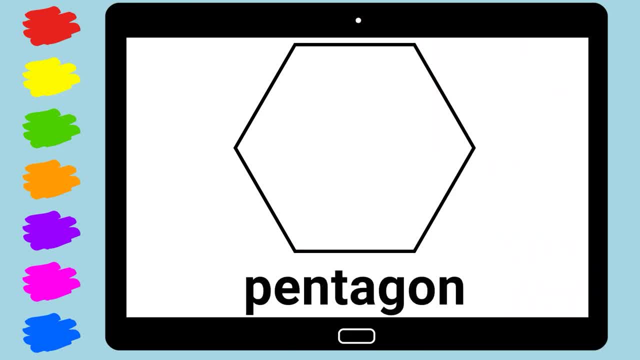 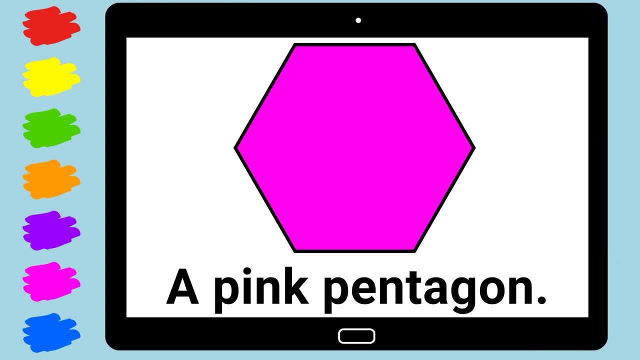 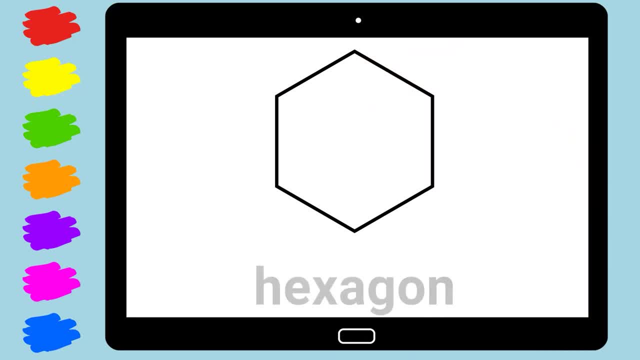 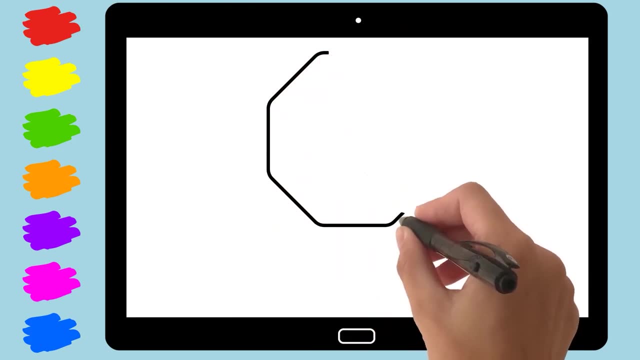 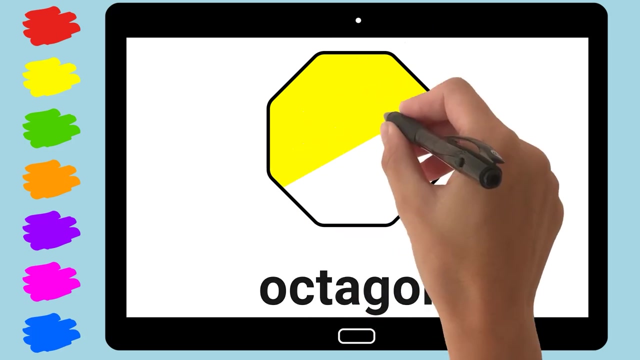 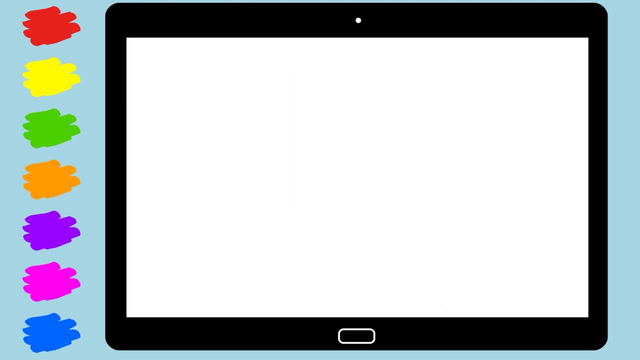 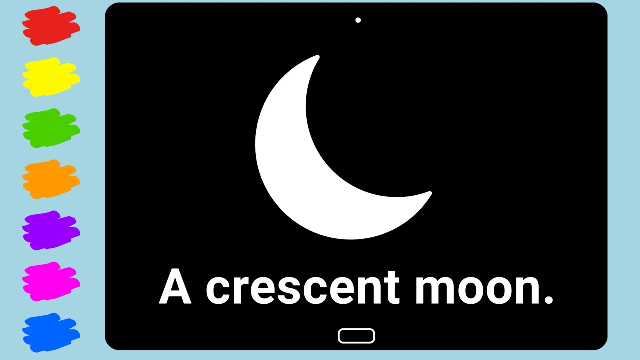 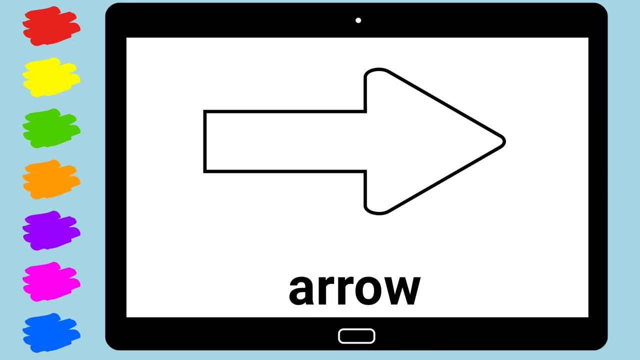 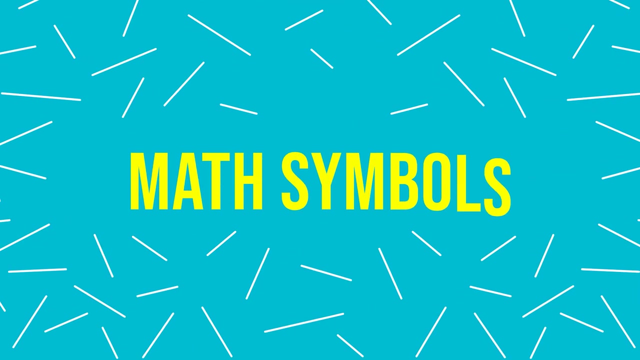 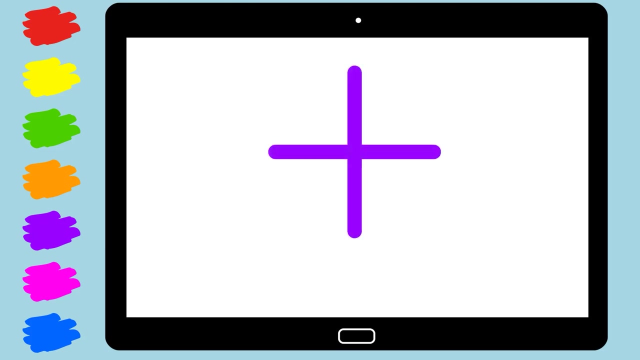 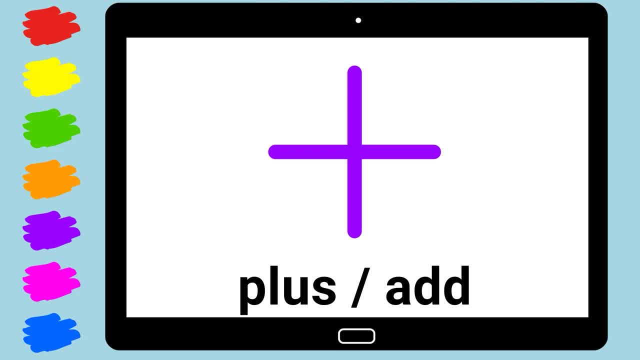 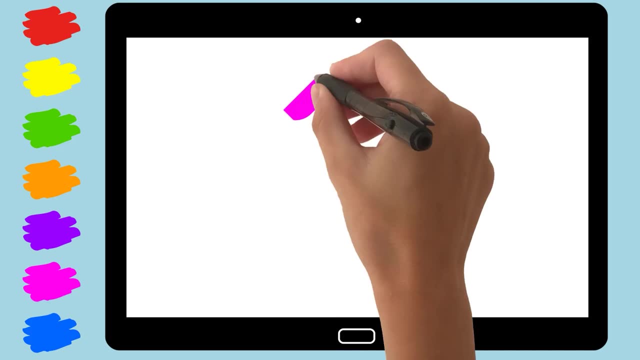 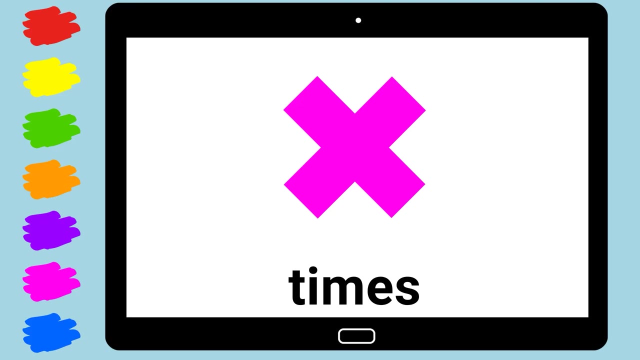